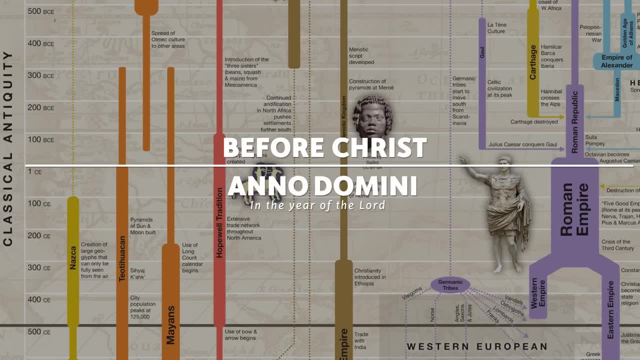 to BC. the dates start going back up, And I should point out that there is no year 0. So, basically, the year 1BC was followed immediately by the year 1AD. Nowadays it's becoming more and more standard for historians to use the terms CE and BCE instead. CE stands for: 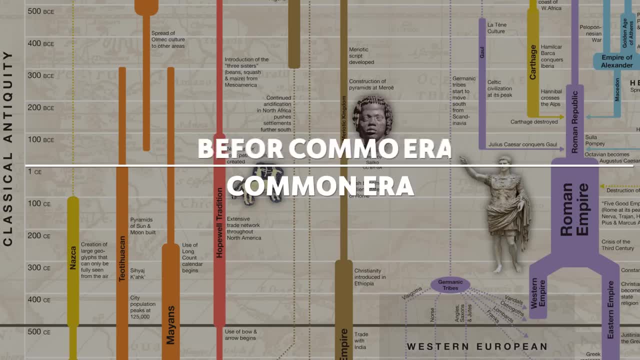 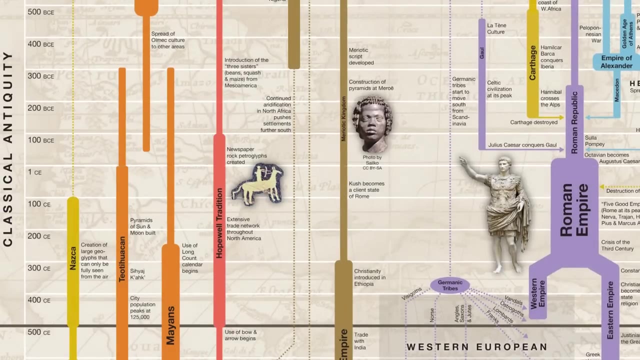 Common Era, and BCE stands for Before the Common Era. The reason for the change is simply an attempt to use a more neutral term, which makes sense considering that 75% of the world is not Christian. Okay, now that we've got that under our belt, the next question we need to address. 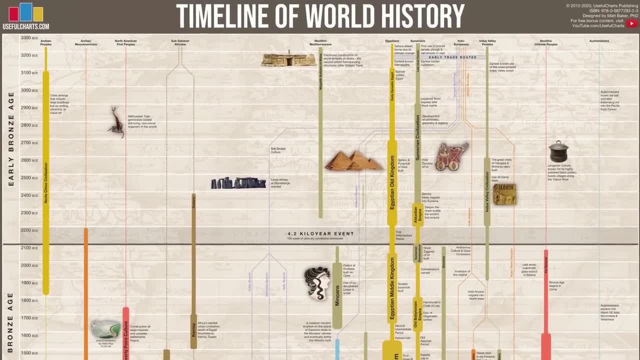 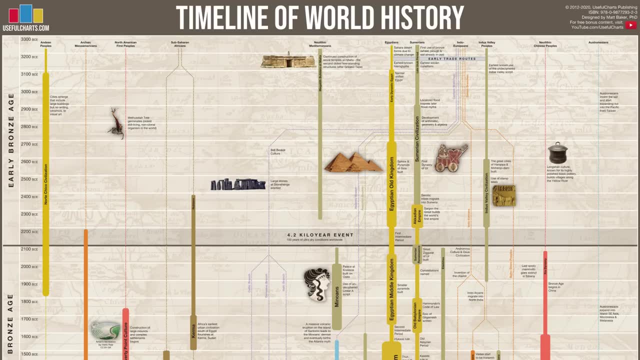 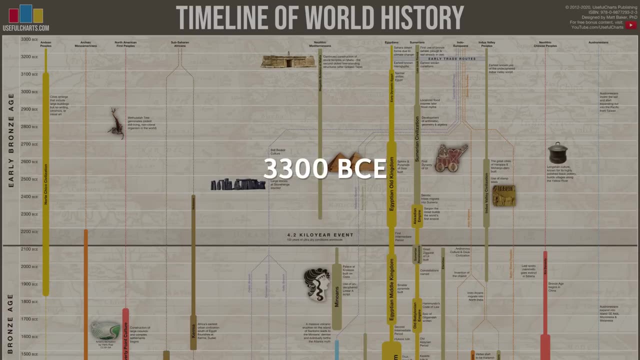 is: what is the starting point for history? In other words, where do we draw the line between history and prehistory? Well, on this chart, I've used the year 3300 BCE as my starting point. The reason for this is that this is approximately when. 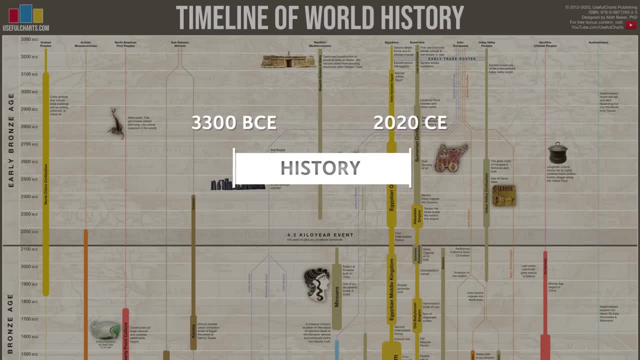 writing first appeared. The basic idea is that without written records we can't have history. Therefore, everything before the emergence of the first writing systems is best categorized as prehistory. And, of course, prehistory goes back much farther than 5300. 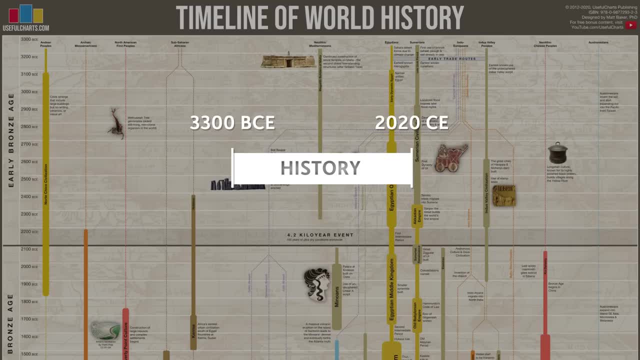 years. So if we talk about the prehistory of our species, Homo sapiens, it goes back about another 200,000 years, a time period also known as the Stone Age. And if we're talking about the prehistory of the planet Earth, well, that goes back about 4.5 billion years. 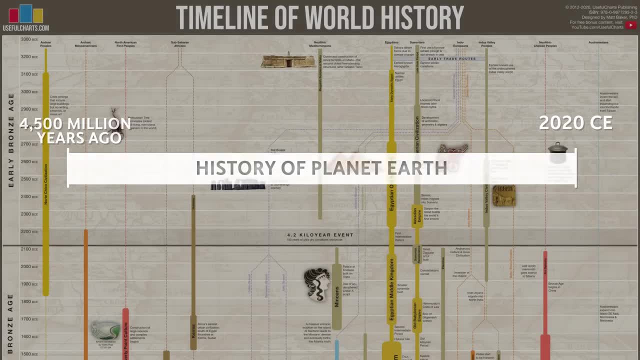 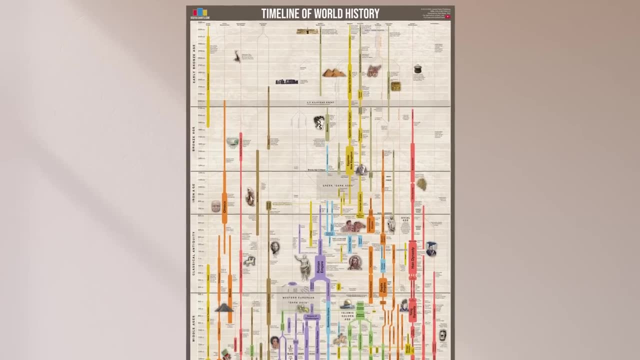 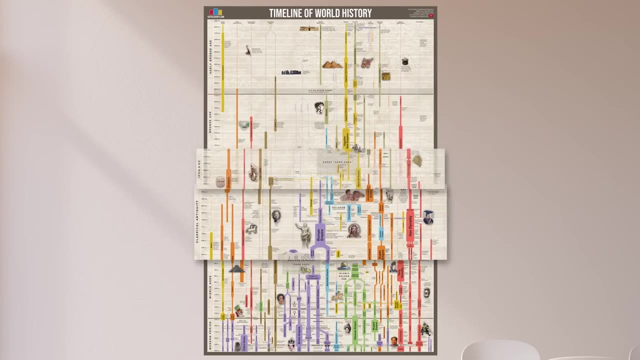 But this chart doesn't cover prehistory. Instead, it starts with the emergence of written records and goes from there So on this chart, history is divided into six main time periods – the Early Bronze Age, the Bronze Age, the Iron Age, Classical Antiquity. 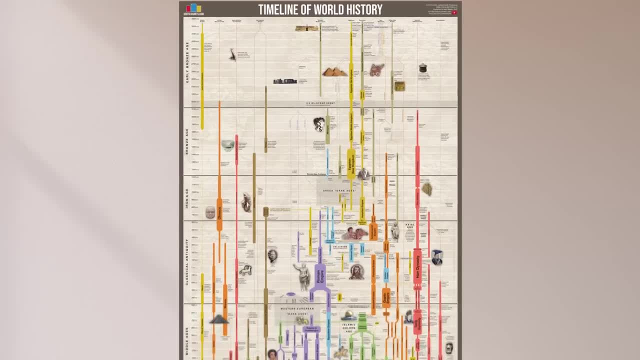 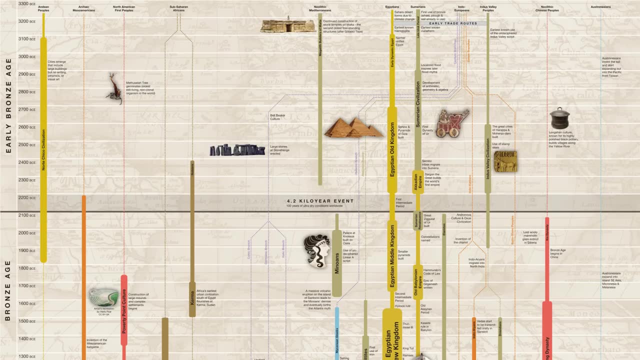 the Middle Ages and the Modern Period. Let's now take a look at each one by one. The Bronze Age gets its name based on the fact that humans first started to make things out of bronze around the same time that they first developed writing. This occurred in: 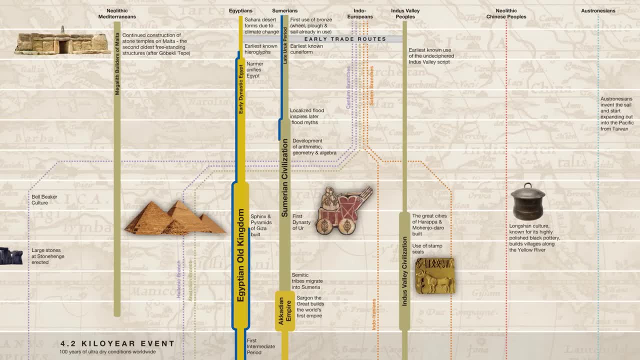 three main areas – Egypt, Sumer and the Indus Valley. modern-day Pakistan. Unfortunately, the writing system used in the Indus Valley is yet to be deciphered, so we can only read the records from Egypt and Sumer, But we do know that these three 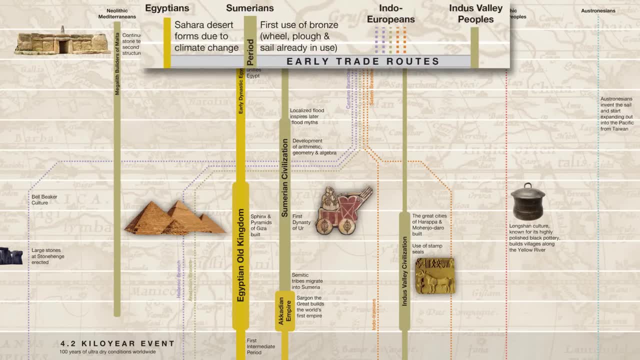 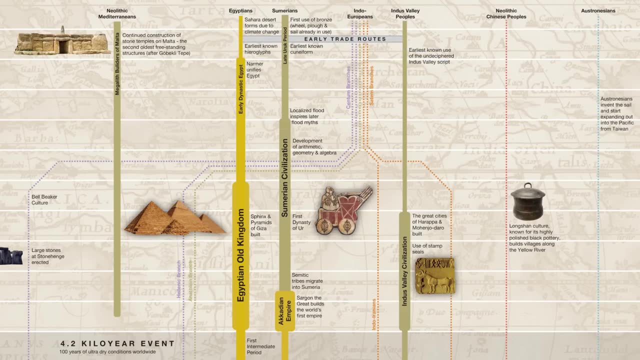 civilizations did trade with one another and that throughout the Early Bronze Age, each grew in terms of both size and technology. At the start of this period, the Sumerians had already invented the wheel, the plow and the sail, But during the Early Bronze 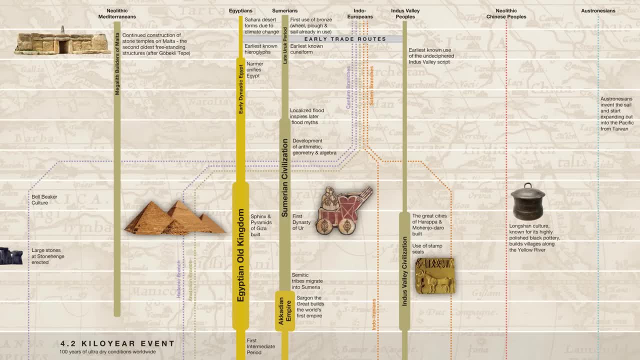 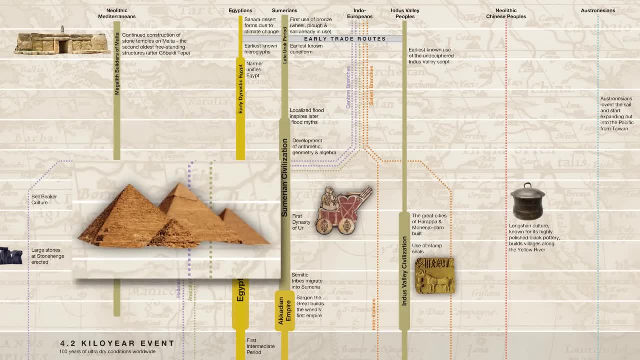 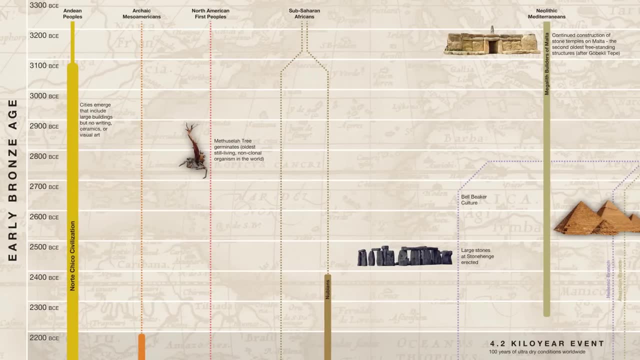 Great Pyramids of Giza were built. Besides these three civilizations, the only other place in the world to have large cities was over in what is today Peru. There, a culture known as the Norte Chico civilization was thriving, But strangely, although they built, 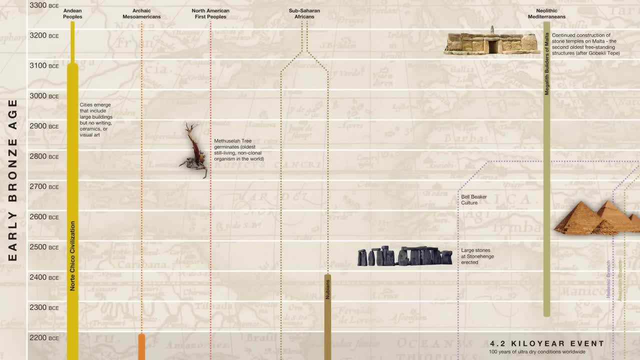 large stone structures. they appear to have had no writing system and no pottery. Stone structures dating from the early Middle Ages were built in the early Middle Ages, and the structures dating from the Early Bronze Age can also be found at Stonehenge in England. 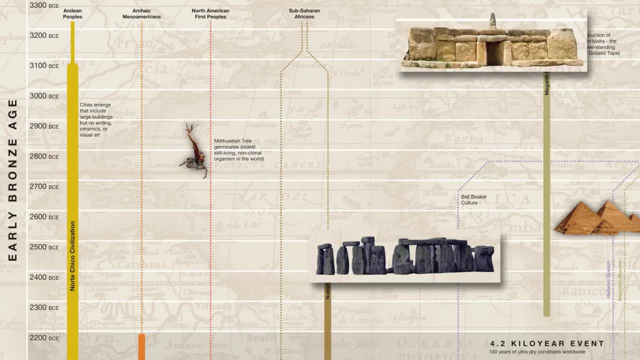 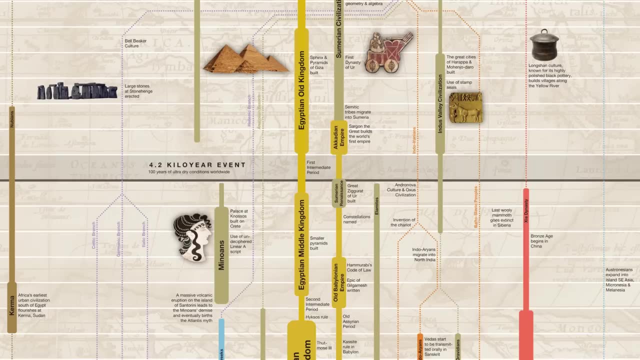 and on the island of Malta, But neither of these places had large populations. Okay, so that was the Early Bronze Age. Now let's look at the Bronze Age proper. Dividing these two time periods is a very important event, known as the 4.2-kilo-year. 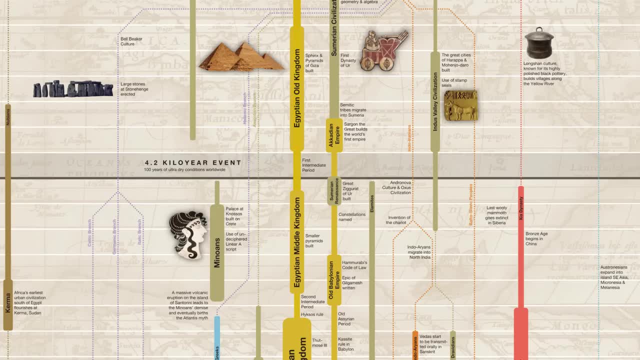 event named because it occurred approximately 4.2 thousand years ago. The exact cause of the event is still debated, but what we do know is that it resulted in approximately 100 years of extremely dry conditions worldwide. Because of this, the Egyptian Old Kingdom 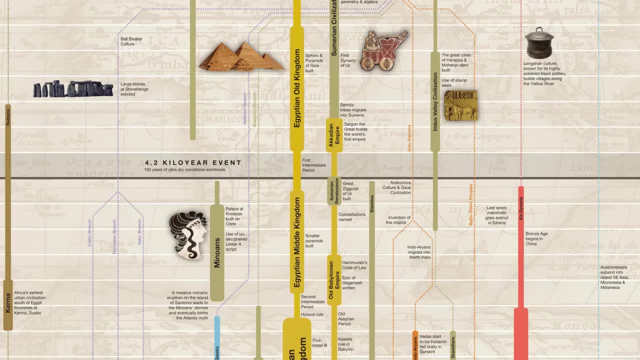 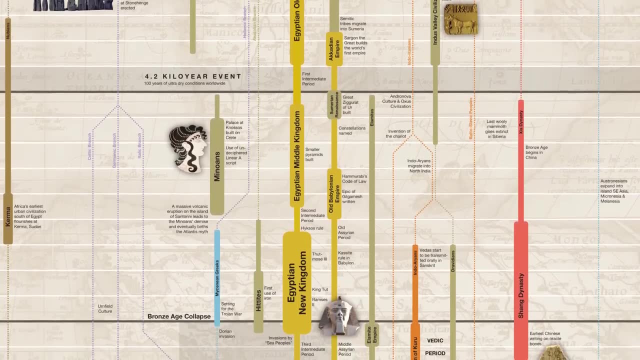 the Akkadian Empire and the Indus Valley. civilization all declined rapidly and in the time period that followed we get a new set of branches. Egypt was revived as the Middle and New Kingdoms, scripo, aeterno and隻bbits. 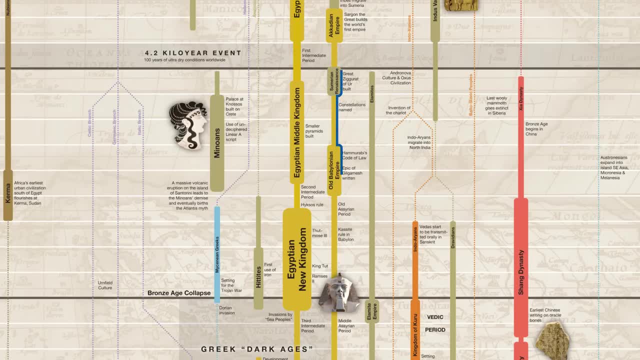 civilization eventually evolved into the Babylonian civilization. But in South Asia we get a more dramatic change. The Indus Valley cities disappear altogether and we get a new set of people arriving, the Indo-Aryans who were part of the larger Indo-European group. 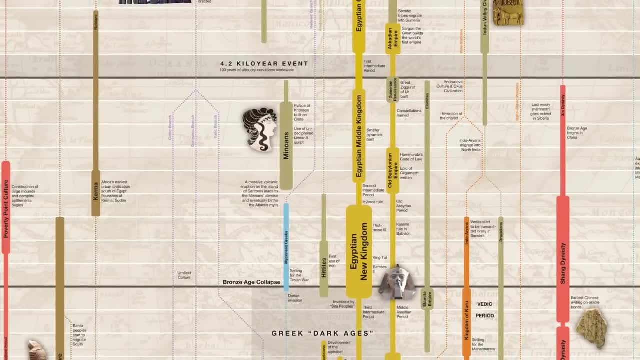 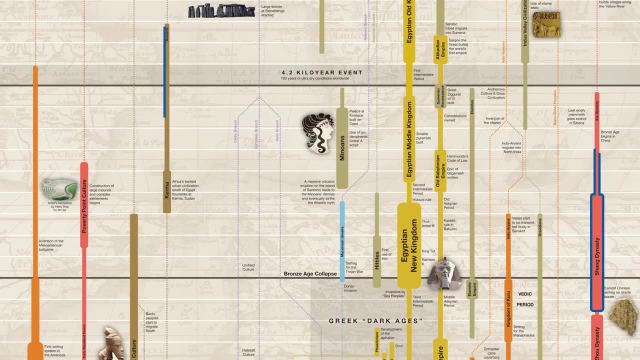 During the Bronze Age proper. we also get civilizations arising in other parts of the world for the first time, including in China, Sub-Saharan Africa and- unbeknownst to many people- North America. There we get the Poverty Point culture where large mounds and complex 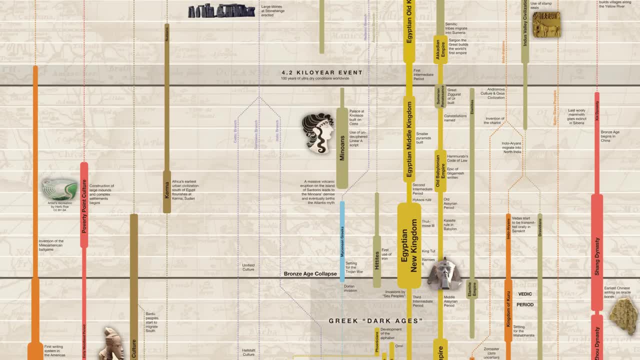 settlements were built. Finally, we also get the first civilization in Europe, the Minoans on the island of Crete. Midway through the period, though, there was a volcanic eruption nearby, which led to the downfall of the Minoans and the destruction of the island of Crete. The Minoans were the first civilizations to 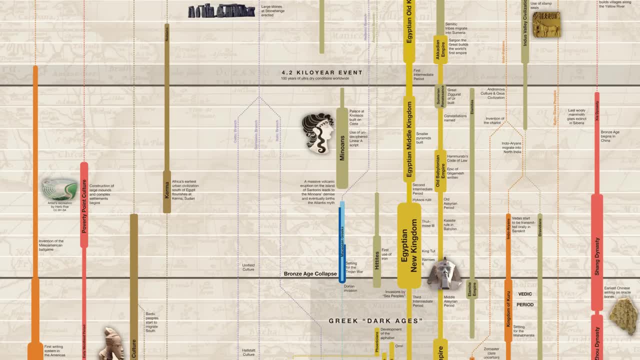 be built in Europe. The Minoans were the first civilizations to be built in Europe. The Minoans were the first civilizations to be built in Europe. The Minoans were the first civilizations to be built in the rise of the Mycenaean Greeks. instead, This catastrophe could very well have been. 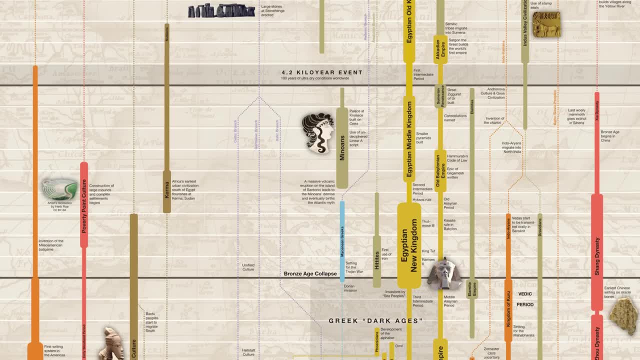 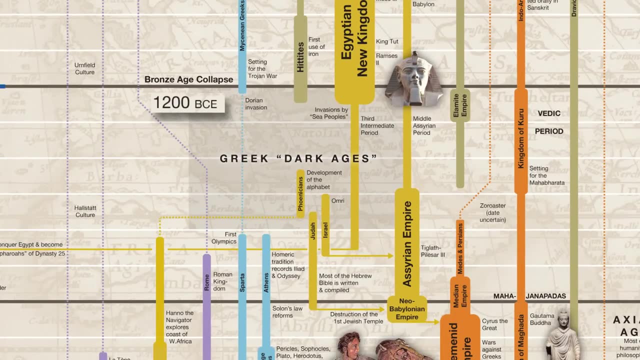 the event that birthed the Atlantis myth. The next big turning point in history occurred around 1200 BCE, and it is known as the Bronze Age Collapse. For reasons that are still somewhat unclear, the major civilizations in Greece, Anatolia and Egypt all disappeared almost instantaneously. What followed is often called 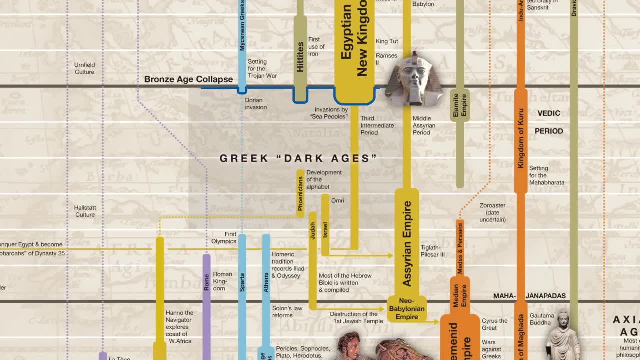 the Greek Dark Ages, a period in which the historical record for the region goes somewhat silent. Interestingly, it is during this silent period that many of the world's most famous legendary tales supposedly took place, such as those found in the Jewish Torah, the Greek. 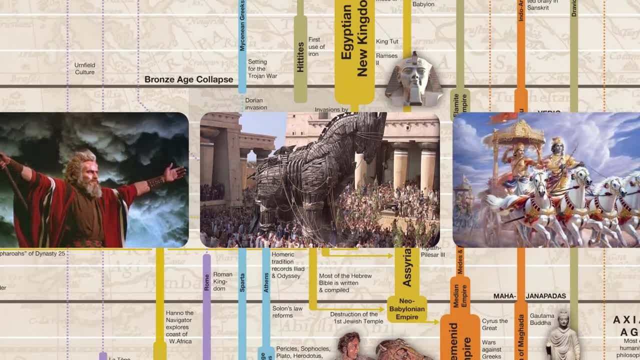 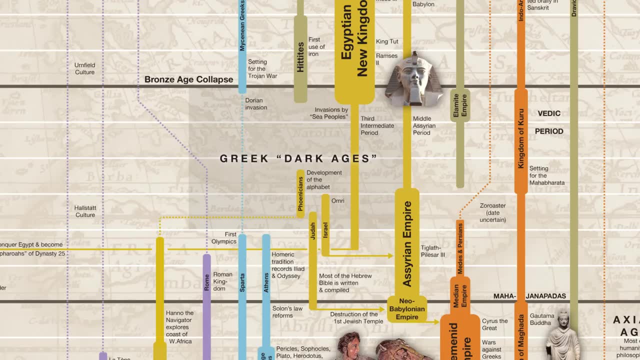 Iliad and the Hindu Mahabharata. The Bronze Age Collapse also coincided with the first use of iron in the Middle East. Therefore, the period in which the Greek Dark Ages took place is also aptly called the Iron Age. This is the third and final. 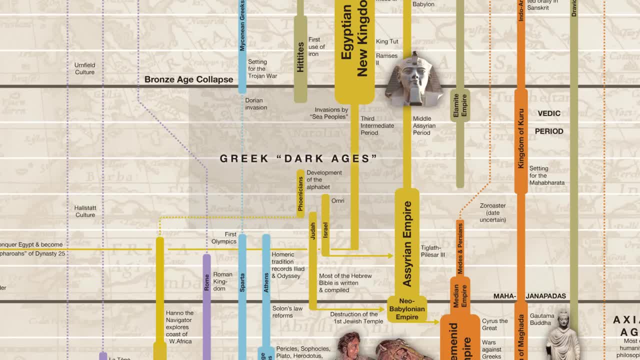 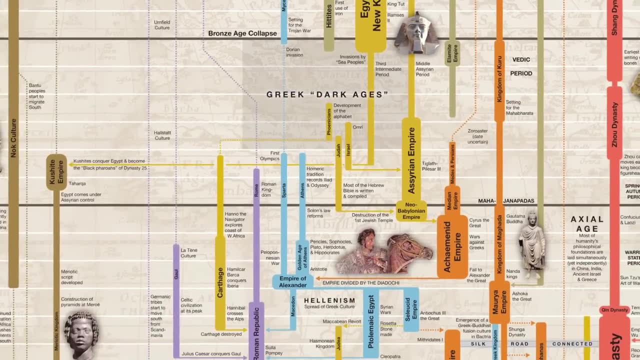 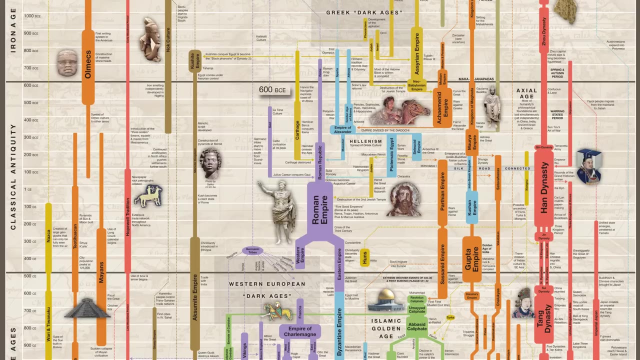 period in what is known as the Three Age System, consisting of the Stone Age, the Bronze Age and the Iron Age. The next period is not actually part of the Three Age System. This is because, after approximately 600 BCE, we no longer have to rely entirely on archaeology to get 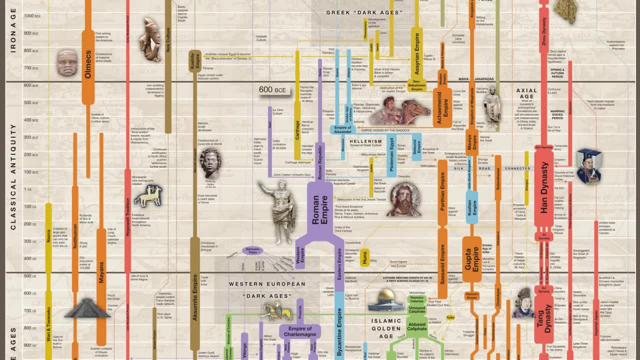 information. As I mentioned earlier, humans have been writing since 3300 BCE, But there is nothing surviving from the Bronze Age or Iron Age that could really be considered a history book. Sure, we have the names of kings, lists of battles. 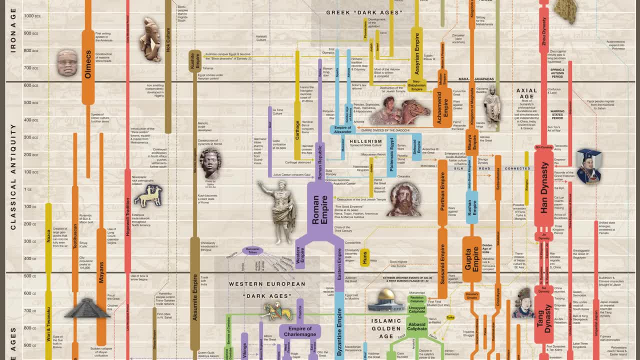 and other details carved into rock and metal, But we don't have anything that starts with. In this treatise I am going to record the complete history of X, But around this time we do start to get such writings, For example from a Greek guy named Herodotus, who is often called the Father. 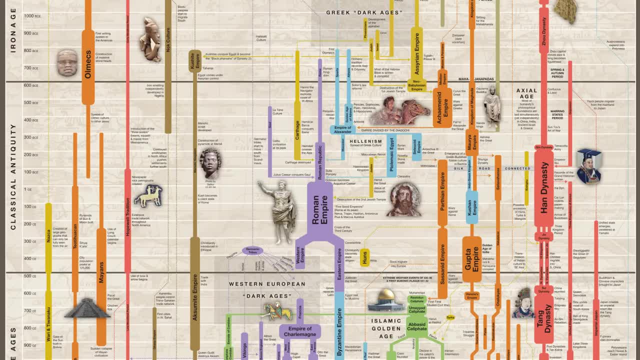 of History. So, in other words, we know a heck of a lot more information about this next period, called Classical Antiquity, than we know about the previous periods. Classical Antiquity is when the Greeks and the Romans laid the foundations for what would 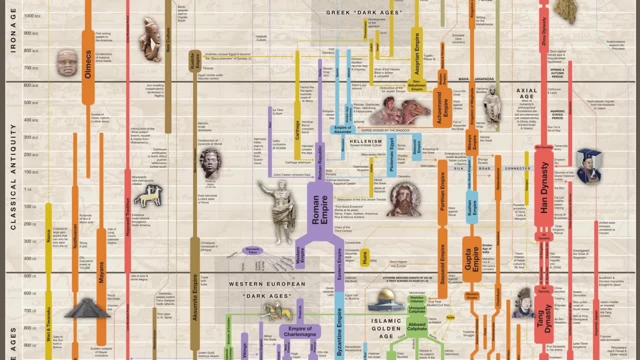 become known as Western Civilization, Mostly by borrowing and building upon information gained from the earlier Bronze Age civilizations. But there was a lot going on in other parts of the world as well. For example, in Mesoamerica, Olmec culture would. 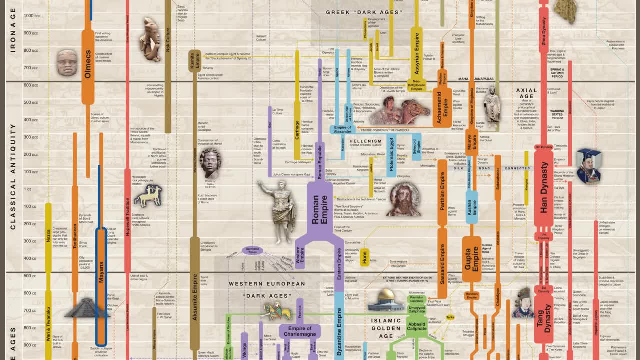 go on to influence Classical Mayan culture with its intricate calendar and writing system, And in North America there was an extensive trade network where lots of different types of art was being exchanged. In Africa, the long-standing Kingdom of Kut Khush eventually gave way to the Kingdom of Aksum. in Ethiopia, There was also the three 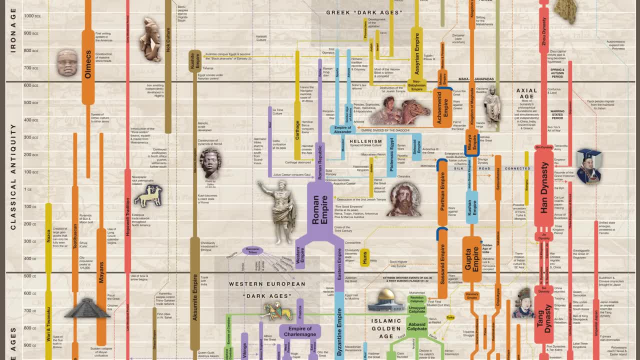 mighty Persian Empires, the Maurya and Gupta Empires in India and the first Imperial Dynasty in China. Eventually, a trade route between all these areas opened up, known as the Silk Road, and thus the western parts of Eurasia and the eastern parts of Eurasia were connected. 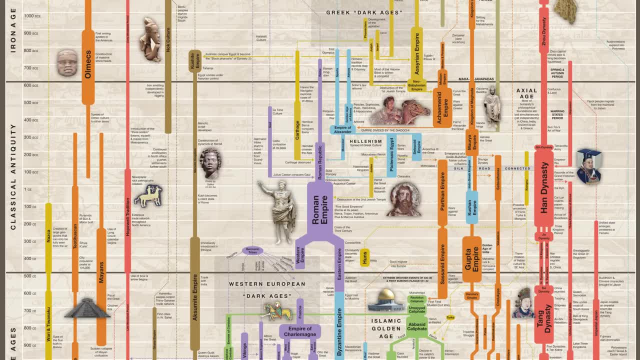 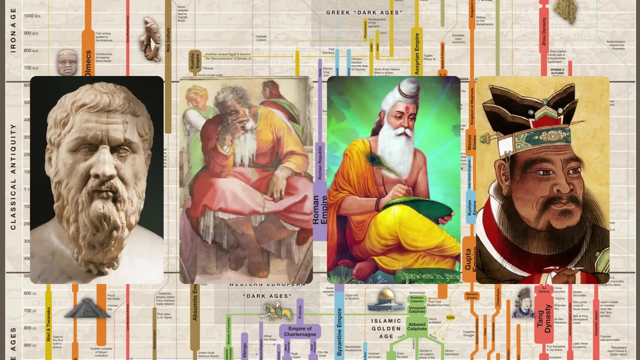 for the first time, But perhaps even more importantly, the time when humanity's current moral and philosophical foundations were laid, Simultaneously yet independently. we got Greek philosophy, the Bible, the Hindu and Buddhist scriptures and the writings of Confucius. We also saw the first experiments with democracy and the 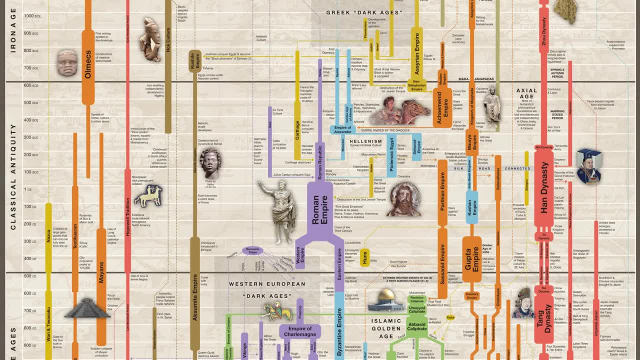 first evidence of truly scientific thinking. But this golden age of human development did not last forever. It came to an end around the year 500 CE with the fall of the Western Roman Empire. In other areas, the classical period ended a little earlier, such as in: 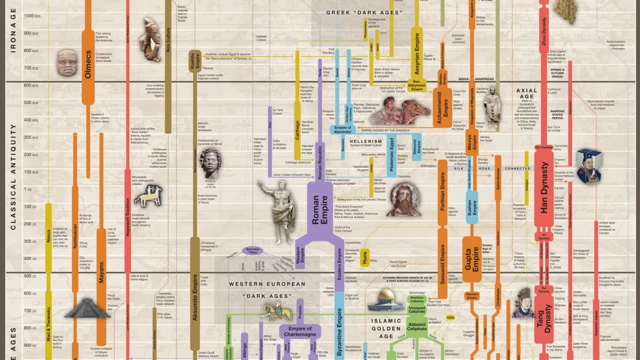 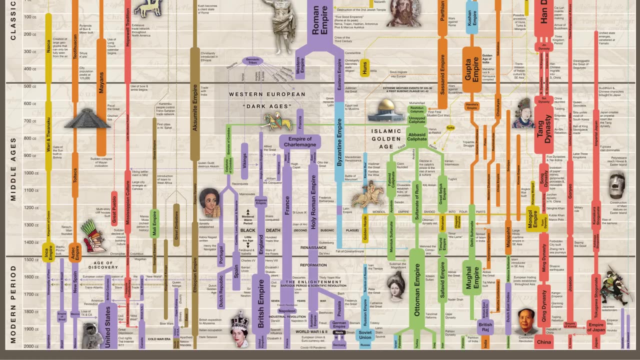 China, or a little later, like in Mesoamerica, But basically all over the world. most of the major classical civilizations eventually crumbled. We then get what's called the Middle Ages. The word middle is used for this period because it is located in the middle between ancient history, which consists of everything we've 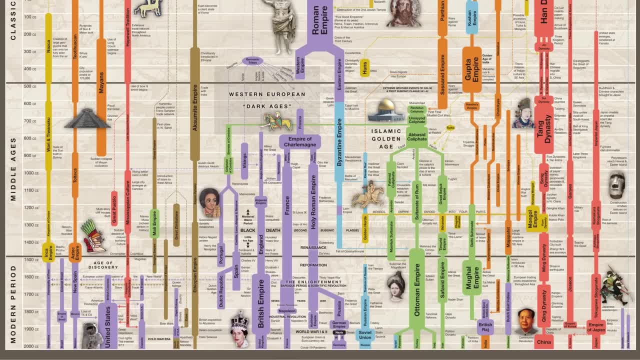 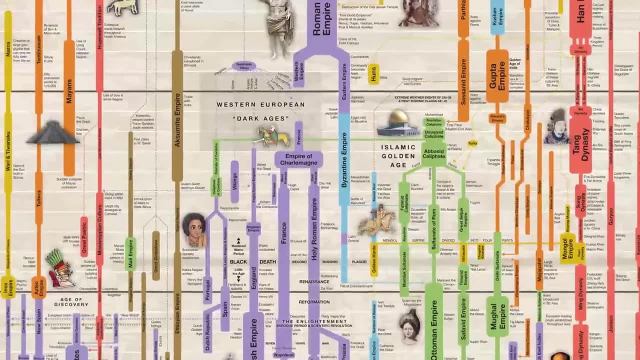 covered so far, and modern history, which we'll be getting to next. It's also called the Medieval Period, Medieval simply meaning Middle Age, But one term that really shouldn't be used for the Medieval Period, but often is, is the Dark Ages. The reason for this: 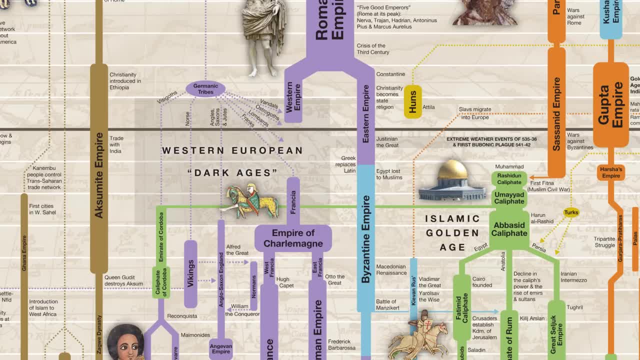 is that the so-called Dark Ages were really just limited to Western Europe. Other areas, such as the Middle East and China, were actually experiencing new golden ages. So what made things in Western Europe change so drastically? Well, numerous theories have been put forward, but one thing we know for certain is that it involved large-scale migrations. 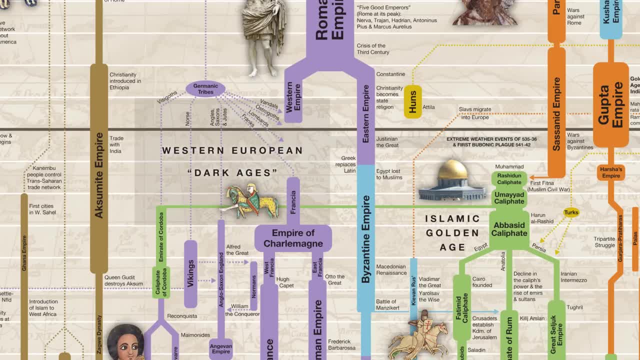 in several parts of the world. Whether or not these migrations were sparked by climate change or some other natural phenomena, we can't be sure, But it ended up creating kind of a domino effect. It ended up creating kind of a domino effect. It ended up creating. 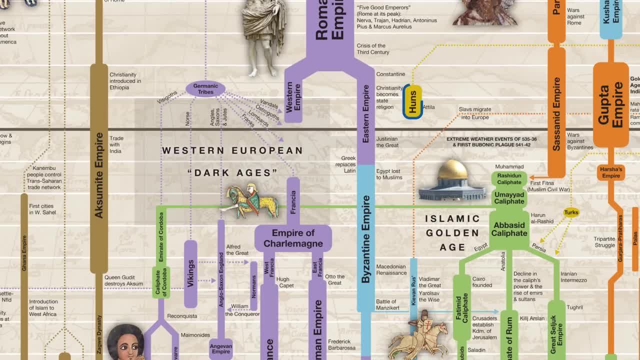 a domino effect. For example, the Huns moved into Europe from the east, and this pushed several Germanic tribes south, bringing them into conflict with Rome. Eventually, it was these Germanic tribes, known to the Romans as Barbarians, who caused the fall of the. 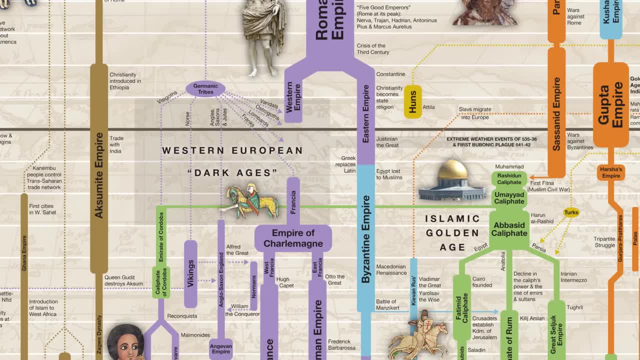 Western Empire and plunged Europe into the so-called Dark Ages. But it wasn't just Barbarians that caused trouble. In the years 534 and 535, the Roman Empire was in a state of total chaos. In the years 534 and 535,, the Roman Empire was in a state of total chaos. In the years 534 and 535,, the Roman Empire was in a state of total chaos. In the years 535 and 536, there were several extreme weather events, perhaps started by a large volcanic eruption that led to famines and cool, dry weather all over the world. There was also the first bubonic plague, also known as the Plague of Justinian, that killed 50% of the population in some cities In the east. these events did not lead to the eastern half of the empire falling, but they did set the stage for the rise of a new civilization nearby – Islam. 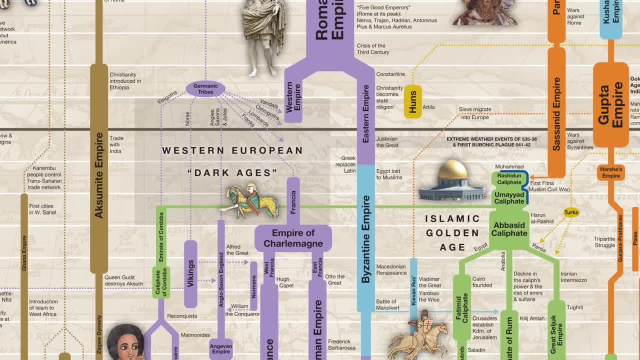 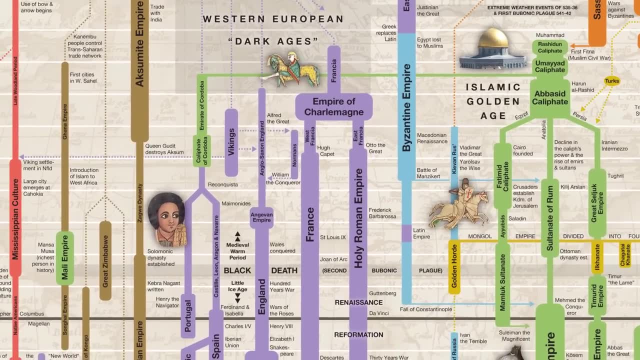 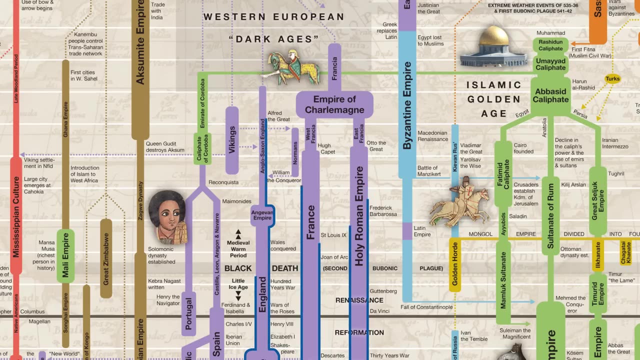 But while Islam was expanding in the Middle East, Christianity was expanding in Europe. Eventually, areas that started out as barbarian kingdoms evolved into major powers such as England, France and the Holy Roman Empire. But there were lots of other things happening in the world during the Middle Ages as well. For example, in West Africa we get several. 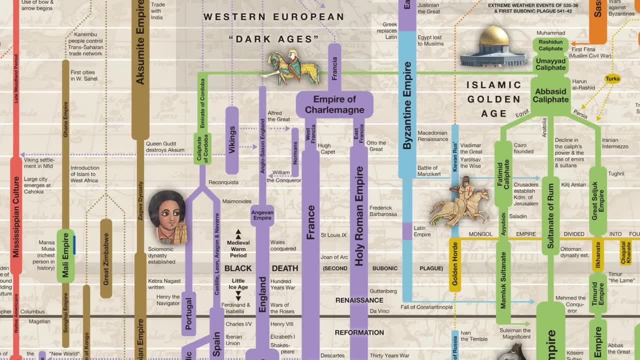 major empires for the first time, including the Mali Empire with its ruler, Mansa Musa, who was the richest person ever in all of world history. And in Southern Africa there was the city of Great Zimbabwe, which included the first large structures ever in that part. 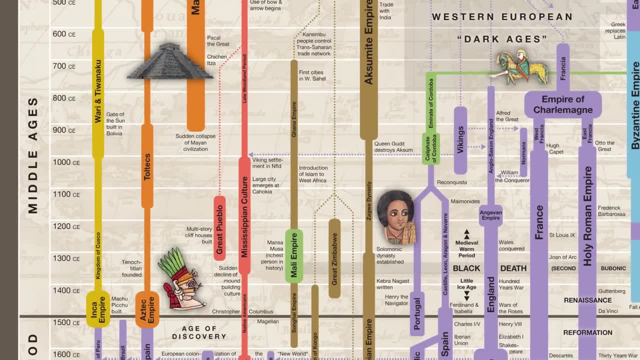 of the world. A lot was happening in the Americas as well. We don't tend to think of cities existing in pre-Columbian North America, but they did. There was Cahokia, the capital of the Arabian Empire, in what is now Illinois, as well as the Puebloan cities in New Mexico, In Mesoamerica. 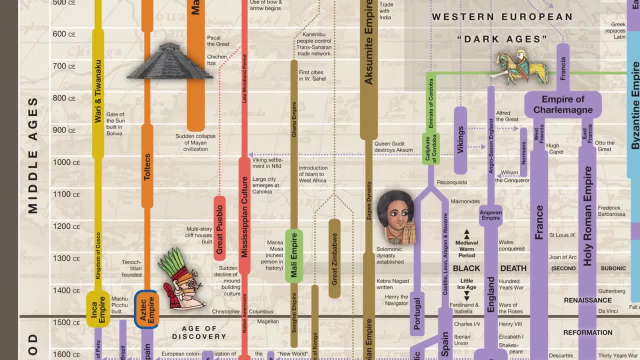 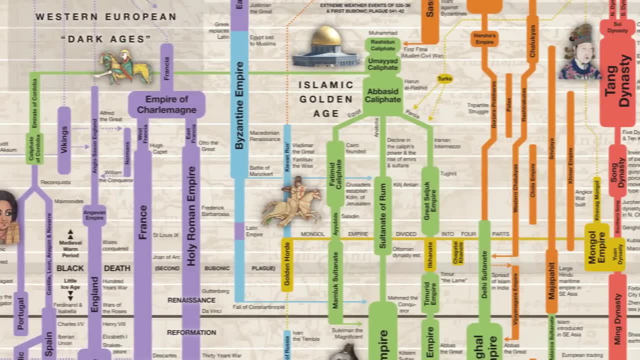 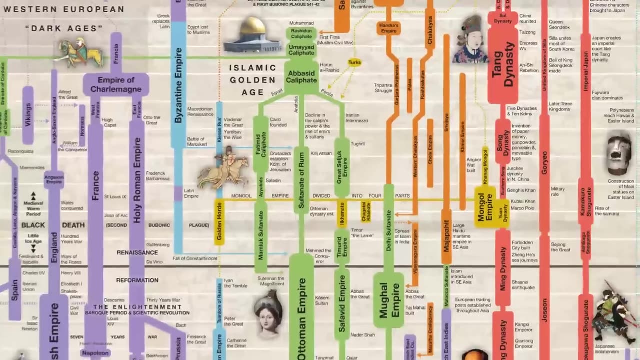 the Aztecs were dominating, And in South America there were the Incas. Finally, it was during the Middle Ages that we get the largest land empire of all time, the Mongol Empire, started by Genghis Khan. Okay, we now come to the sixth and final time period – the Modern Age, which is the 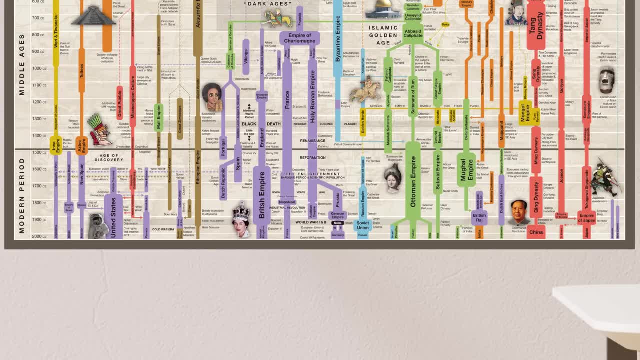 period in which we live today. One could argue that the transition started with the most deadly pandemic of all time, the Black Death, also known as the Second Bubonic Plague. Once again, up to 50% of the population in many cities passed away, and this perhaps helped spark the Renaissance. 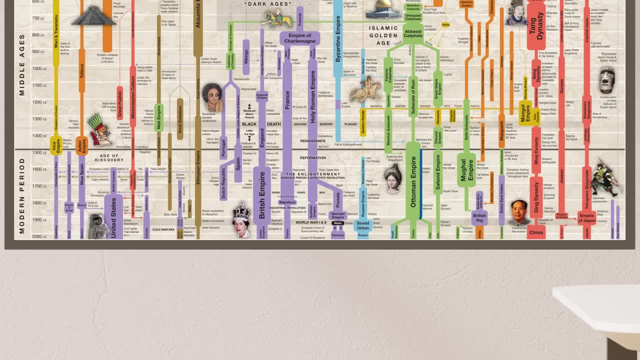 The Eastern Roman Empire finally fell to the Ottoman Turks, and in Italy there was a renewed interest in studying the art and the culture of the Roman Empire. The Roman Empire was a very important part of the European history and philosophy of the Classical Period Around. 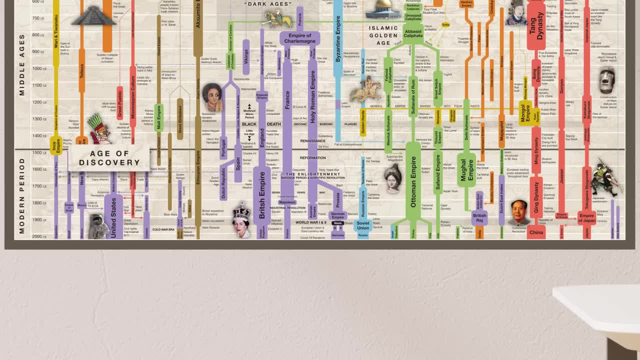 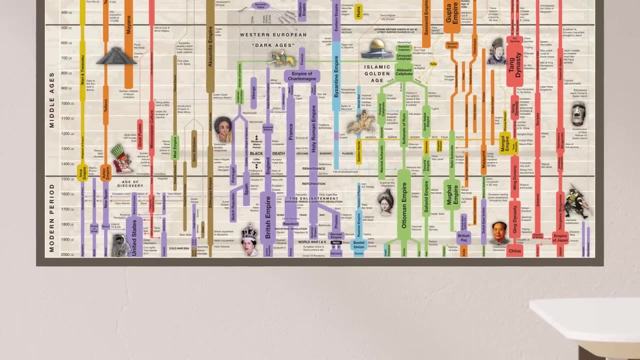 the same time, Europeans started colonizing the Americas and major advances were made in science. This in turn led to the Industrial Revolution, which then gave way to the Technological Revolution which we are still experiencing today. Okay, so that was obviously a very broad overview, But what I think is perhaps most interesting,